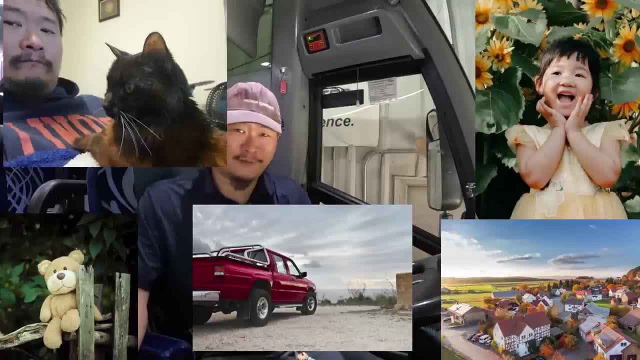 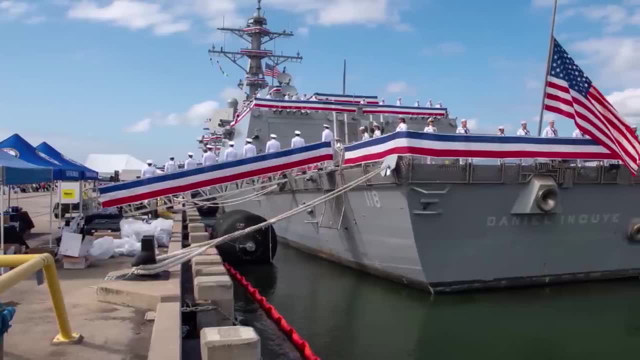 live, as well as our things, including the vehicles that we use to get around. In the old days, ships were given just one simple name. Now, modern day ships not only have a name, but also a registry number or a unique whole number of some sort. 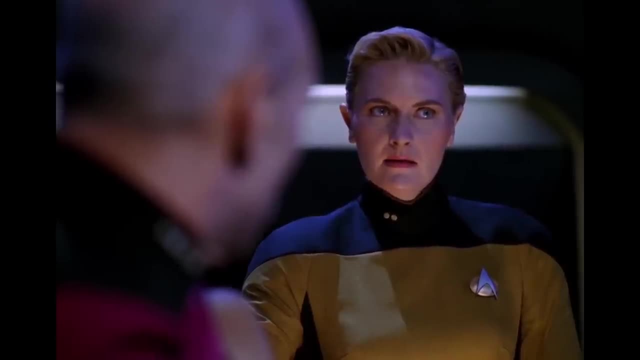 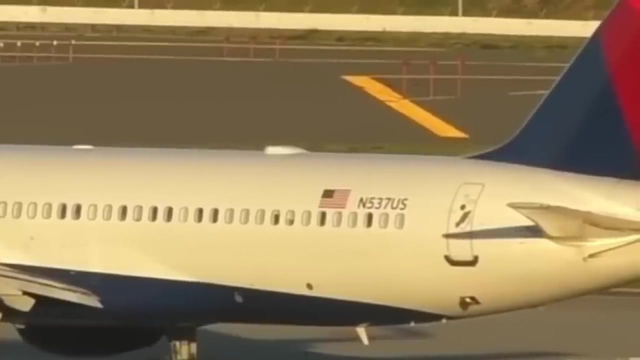 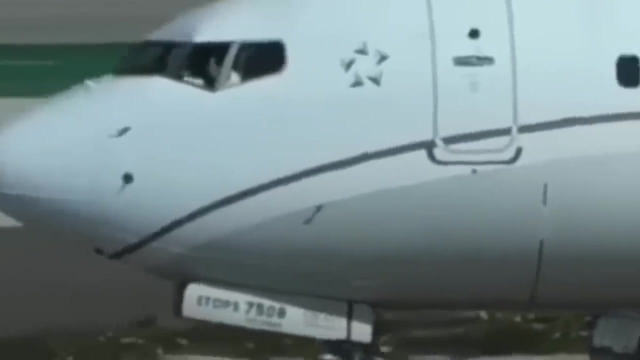 Airplanes are identified by an in number on their tails. usually When purchased by an airline, the airlines usually give them an additional set of fleet numbers, usually a two to three digit number, so that they can recognize all the different aircrafts that they have in their 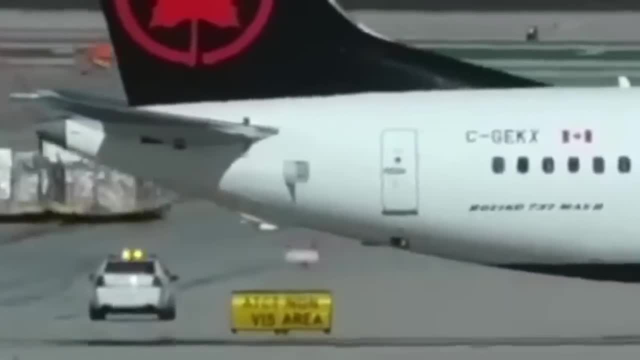 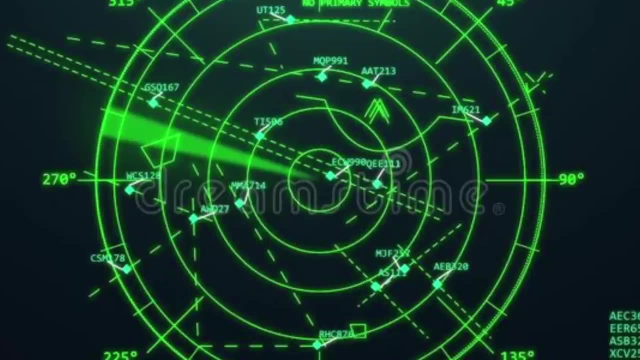 fleet with ease instead of using the long in tail numbers. On top of those two numbers, dispatch also assigns a flight number so that air traffic can be seen. Controllers can recognize them in the air and know where they're going and what they're hauling. 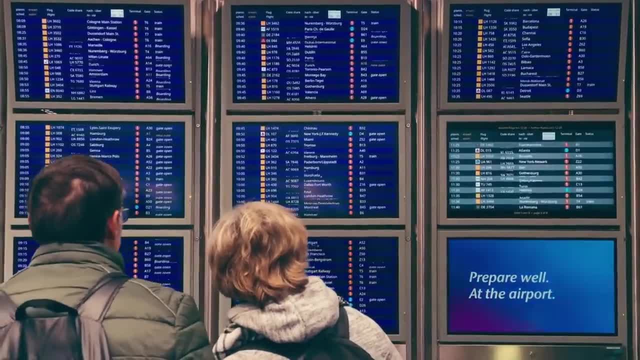 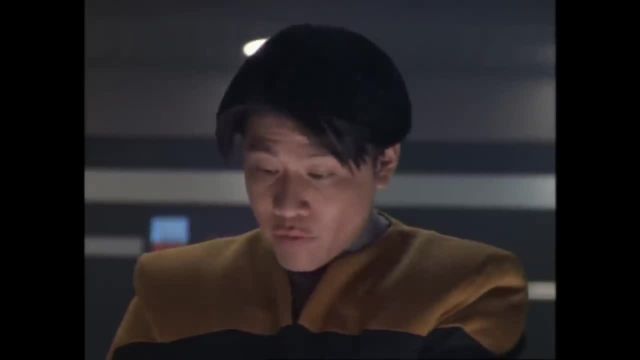 This usually helps passengers as well to know which plane we want to get on, so that we don't end up somewhere that we didn't intend on going to. If these sensors are working, we're over 70,000 light years from where we were. We're on the other side of the galaxy, But what about buses? 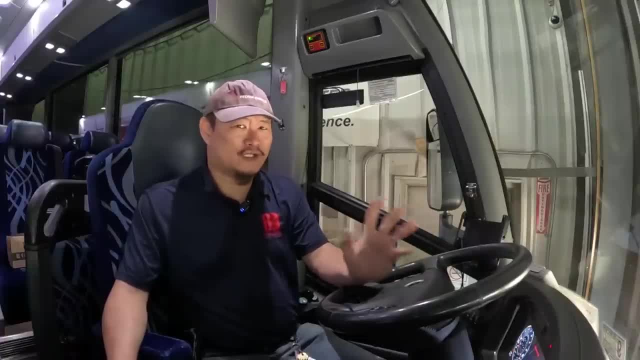 Well, if you look closely, depending on what type of bus it is and what kind of jobs that it does, buses have all kinds of different numbers and identifiers all over the world. So if you look closely, you'll see that there are a lot of different. 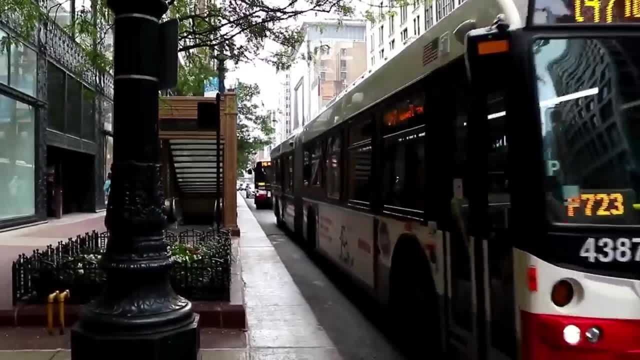 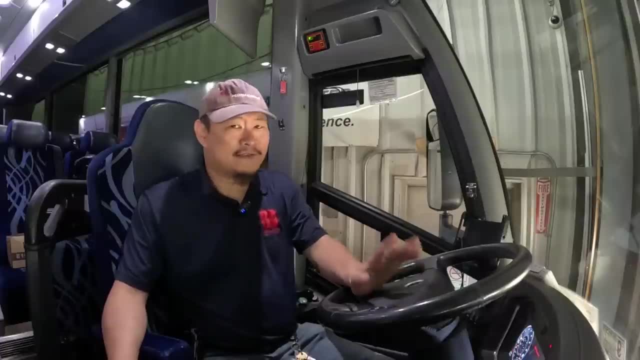 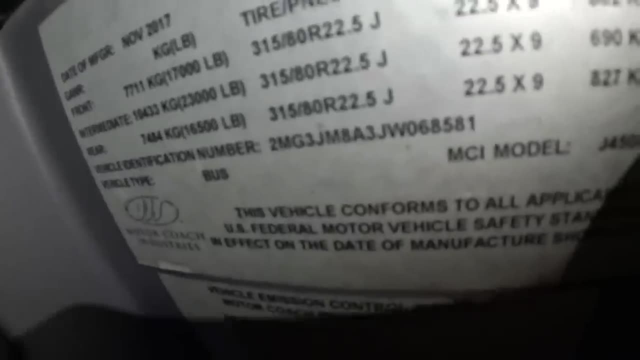 numbers and identifiers all over them. Today, we're going to take a look at just what all these numbers mean, as well as how they get them. Just like personally owned vehicles, all buses have their own VIN numbers. They're typically 17 characters long and they're assigned when they're being built in the factory And they 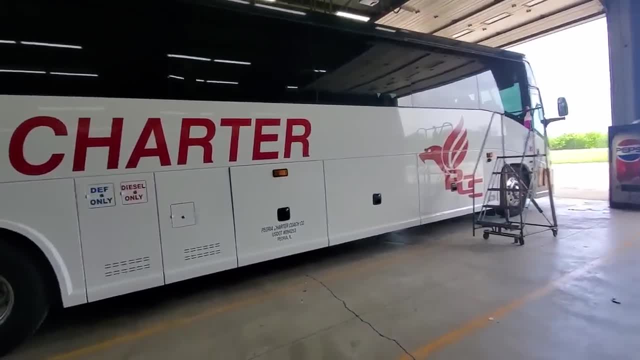 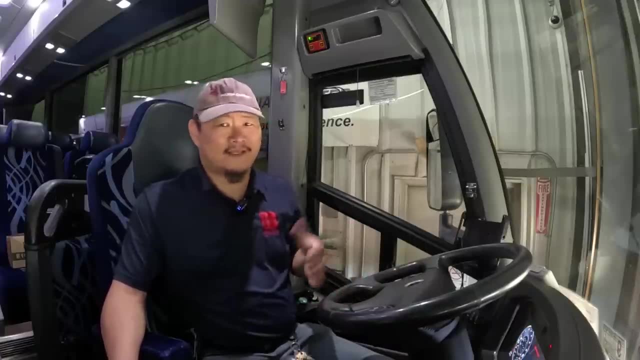 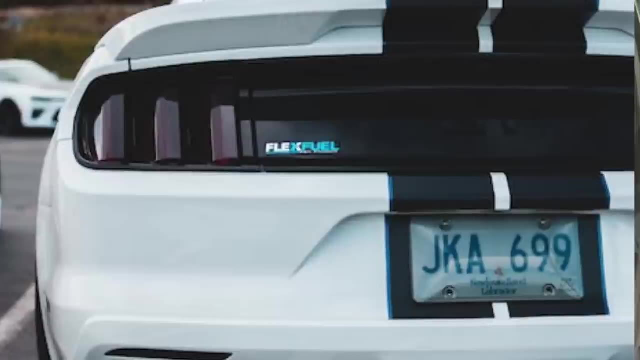 are unique to that vehicle and that vehicle only. But when they're purchased by a company, the company purchasing them have to slap on a few more identifiers before they can send them out for passenger service In North America. the first set of numbers will be the license plate number. Just like buying your own car, you'll need to get a. 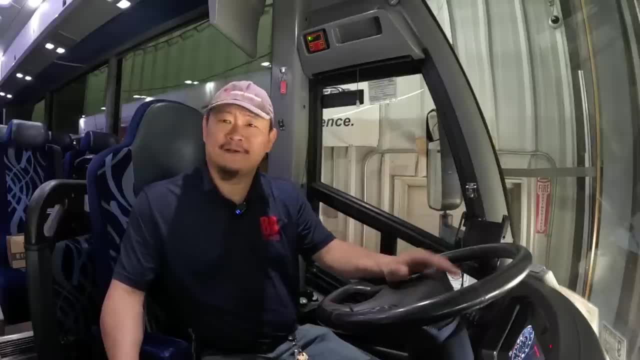 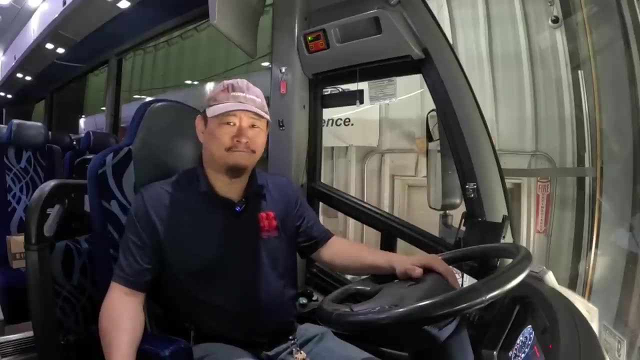 license plate for your bus, But not just any type of license plate. You'll need to get a specialized passenger carrying license plate, And there are lots to choose from, From PT plates for vehicles with a capacity of up to and including nine seats to apportioned plates, which are required for 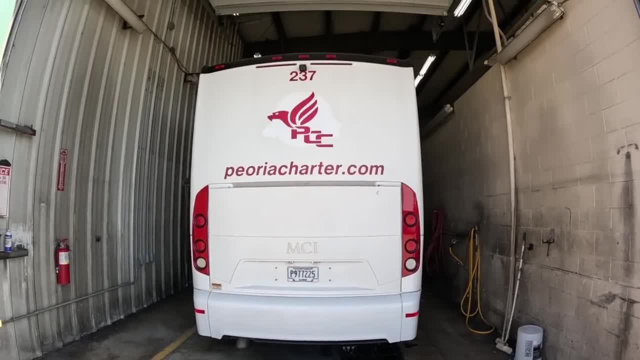 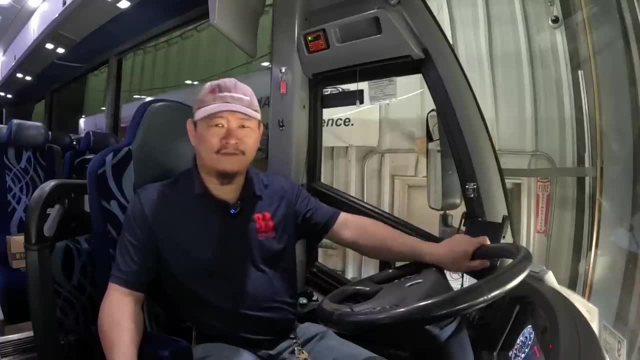 vehicles operating in two or more states, or even more states. So if you're buying a bus, you'll need to get a license plate for your bus. Now, there's a lot to research when choosing what type of license plate you should get for your bus, But since this video isn't about 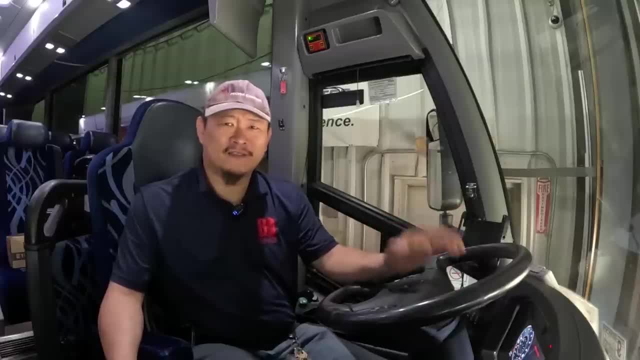 license plates. I'm not going to talk too much about all the different types, But if you guys are interested in a video just about the different types of commercial plates in North America, let me know down in the comments below. It might be worth doing something there. 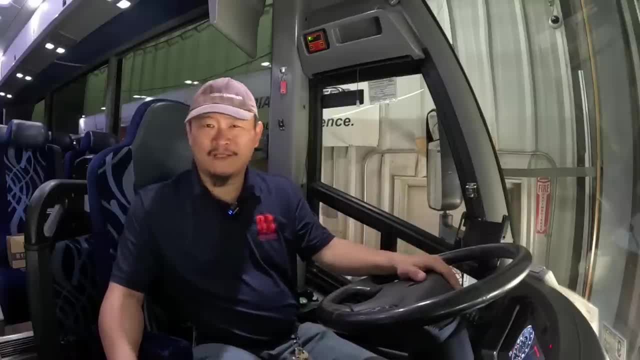 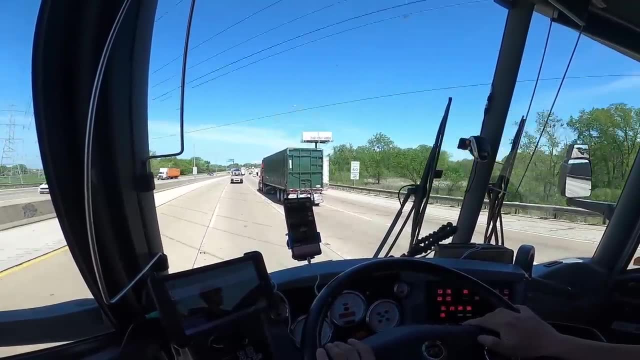 So now, let's say you got your license plate ordeal taken care of. Well, what else? Well, if you operate a motor coach and you plan on taking your license plate to North America, you're going to need to register for a DOT number And, depending on what state you operate, 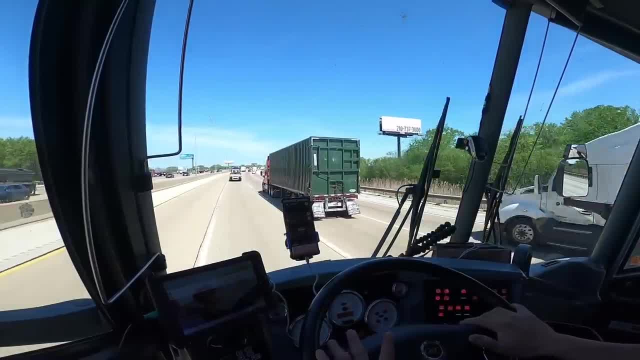 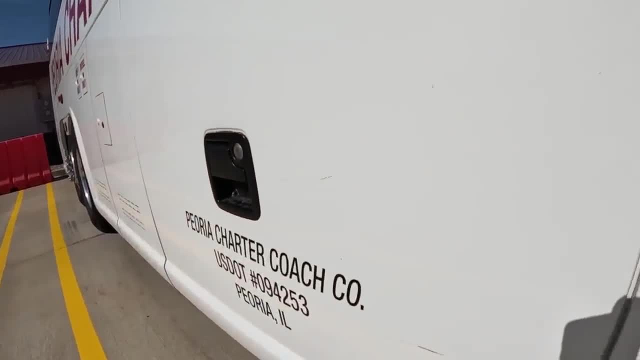 out of you may also need to register for an MC number, which actually used to be called an ICC number. Every commercial truck or coach bus will usually have this number, as well as the name of the company they operate for, either painted or decaled somewhere on the 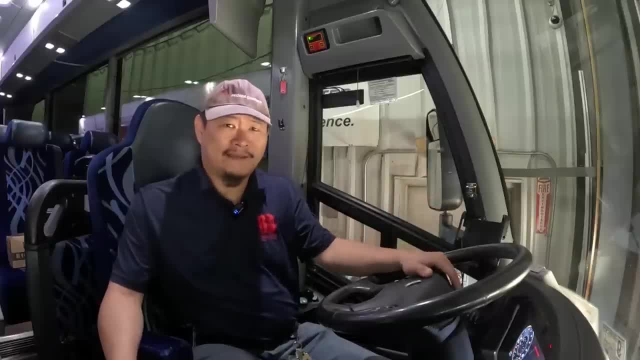 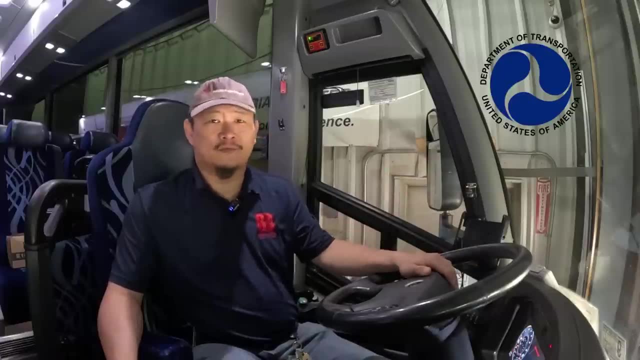 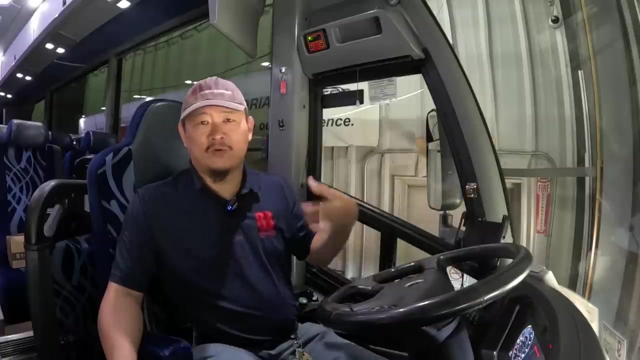 side of the vehicle. These numbers are assigned to your company by the US Department of Transportation. They're unique to the company and is used by the Department of Transportation, or DOT, as well as the Federal Motor Carrier Safety Administration, or FMCSA, to look up your company's information and determine whether. 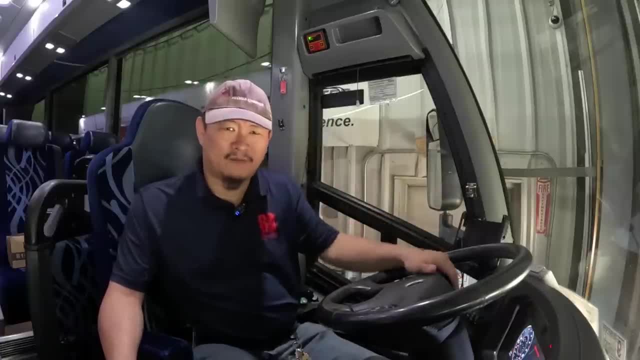 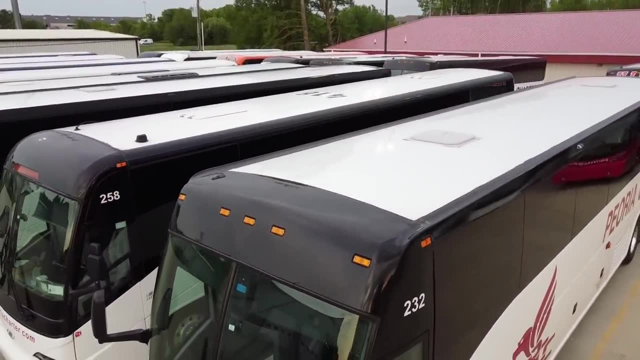 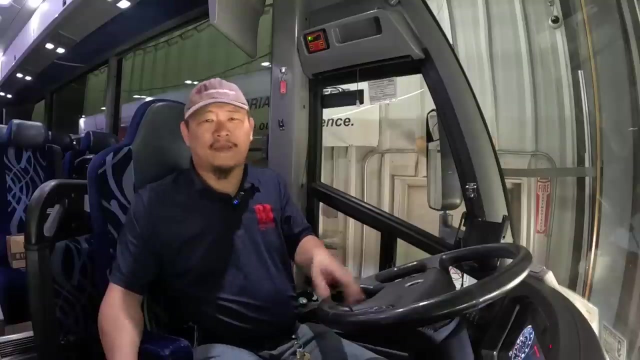 or not you are in compliance. Basically, it's a number for them to check your report card. Whether you own one bus or 100 buses, you will need to obtain these numbers before you start transporting any passengers. Okay, now that we got all the boring and legal stuff. 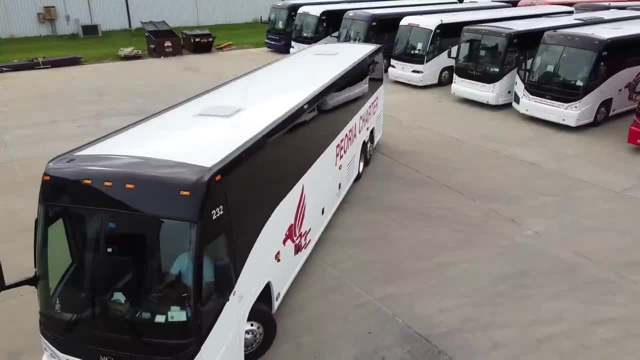 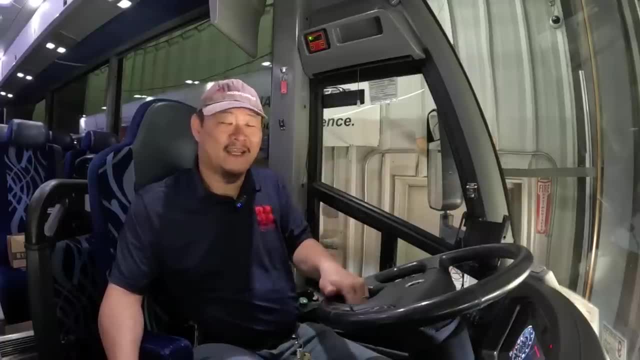 underway. an owner of a commercial coach bus will have the option to give his or her bus a fleet number or, in some cases, a fleet name. In my opinion, this is the best part about getting a vehicle: when you get to actually name it or number it. This is basically what. 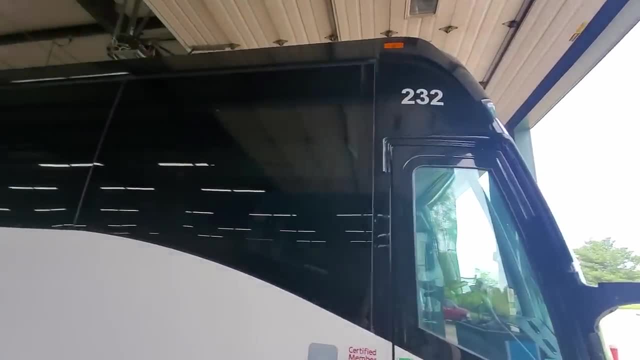 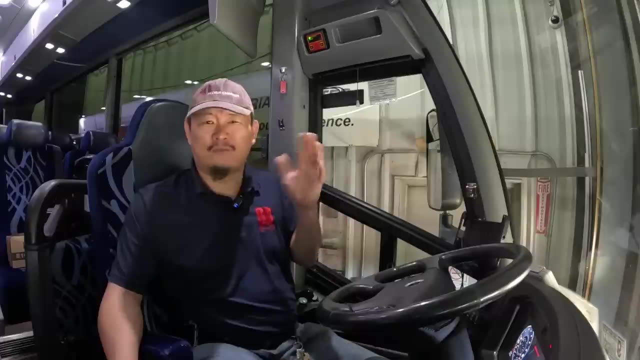 you want to call your coach bus. Now, I'm not aware of any laws or regulations that says an owner of a coach bus has to give his or her coach bus a fleet identifier. Now, if I'm wrong on this, someone please correct me down in the comments below If you are. 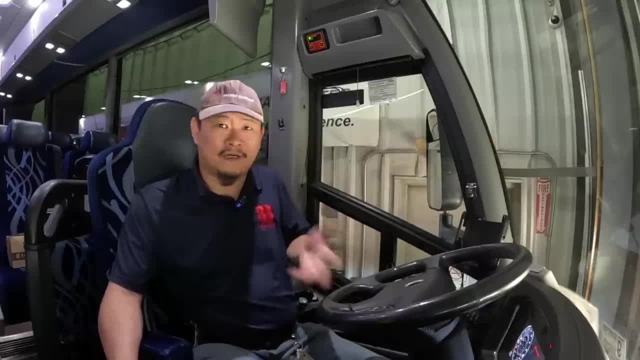 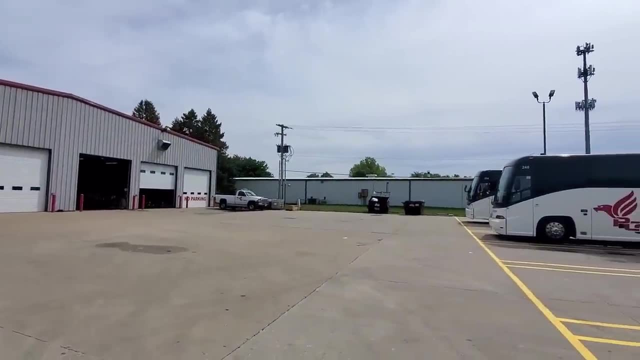 a one bus operation, I guess you really need to have a fleet identifier. So if you're a one bus operation, you really don't need to give your bus any kind of identifier- I mean, unless you really want to- For those who own or operate or manage a fleet of two. 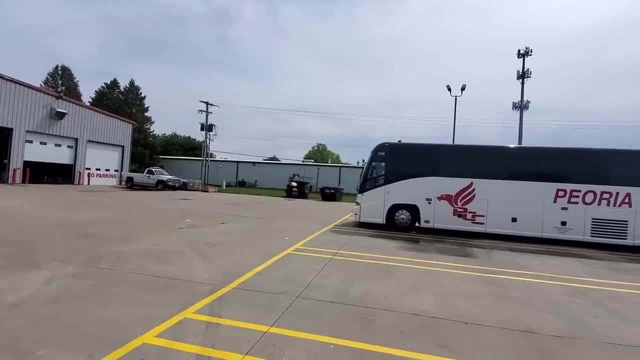 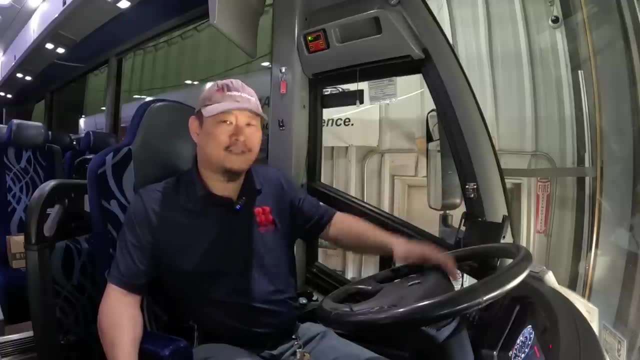 or more buses. if you don't have a way to identify your buses, it could get confusing when you need to assign them to your drivers or if your diesel techs need to go and fix one of them. Then it comes in real handy if you have a way to refer to your buses in your 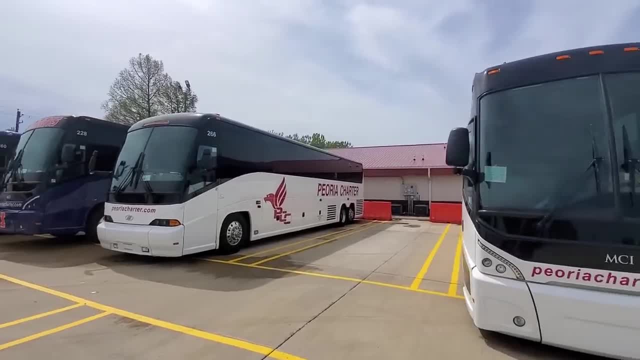 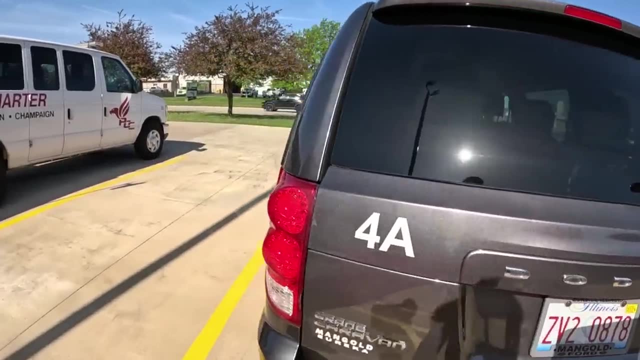 fleet For Peoria Charter, the company that I work for, all of our coaches are identified with a three-digit number And they all start with a two. On our smaller vehicles, like passenger carrying transits or our minivans, they're usually given a single or double-digit number. Now, if you happen, 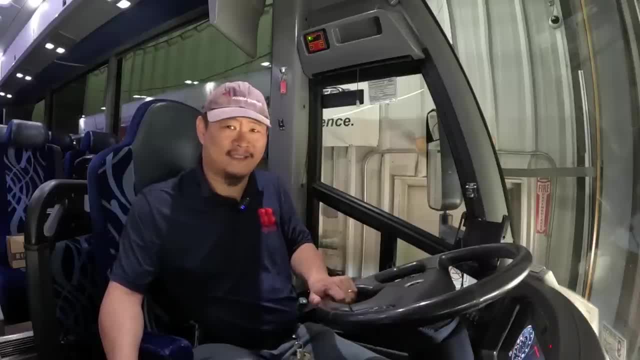 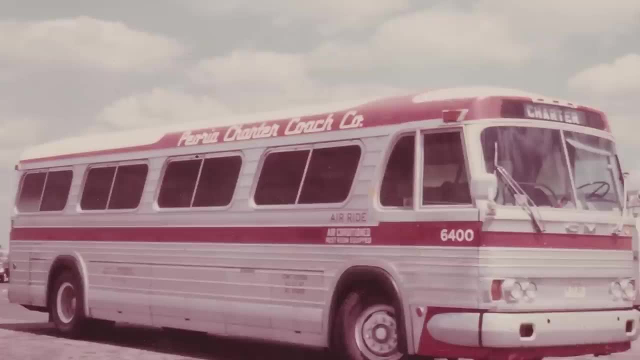 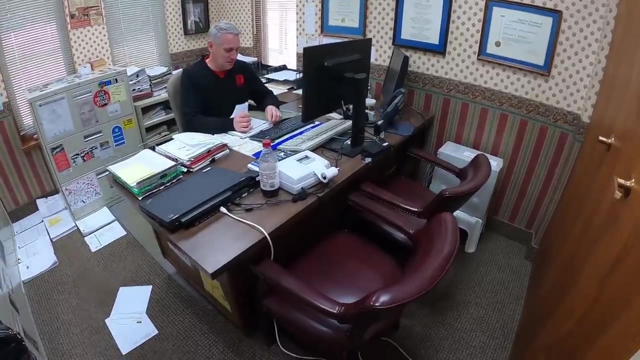 to stumble on some pictures of our buses from way back in the day. they were once numbered quite differently. They had four digits and the first two digits denoted the actual year of when the vehicle was built. Now, in the making of this video, I asked Bill Winkler, the president of Peoria Charter. 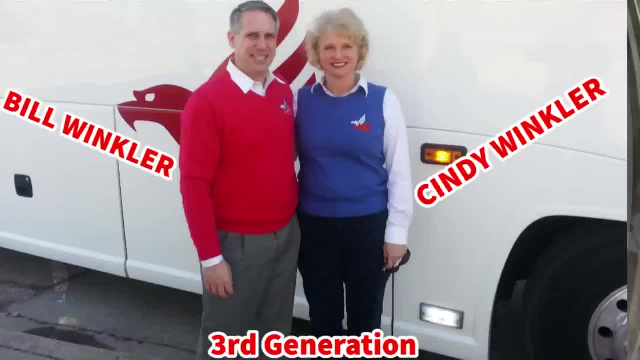 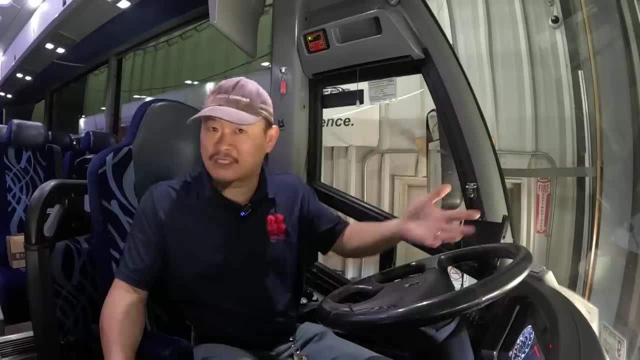 as well as the third generation of the Winkler family to take over the business, why our buses today start with a number two. I mean I always assumed that Bill's father, Roger Winkler, changed the fleet from the four-digit numbers to the three-digit numbers. that now 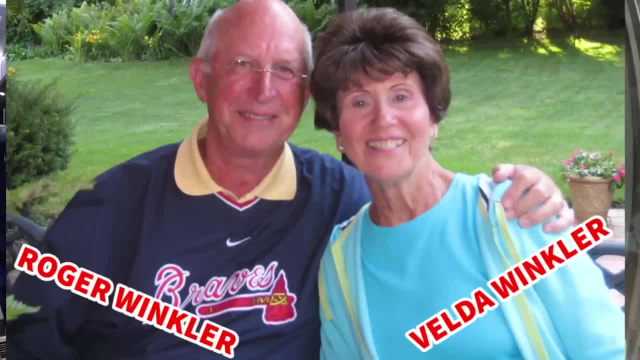 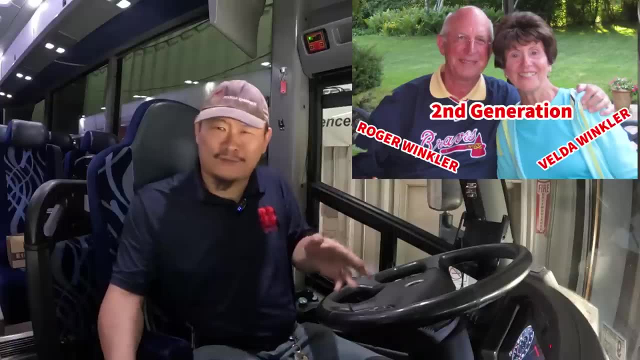 start with the twos, because when he took over Peoria Charter, Roger was the second generation of the Winkler family to run the company, hence the letter two. But that, however, was not the case. Bill actually called Roger Winkler his father. 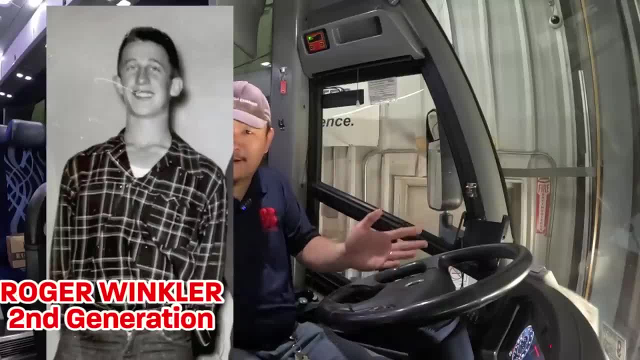 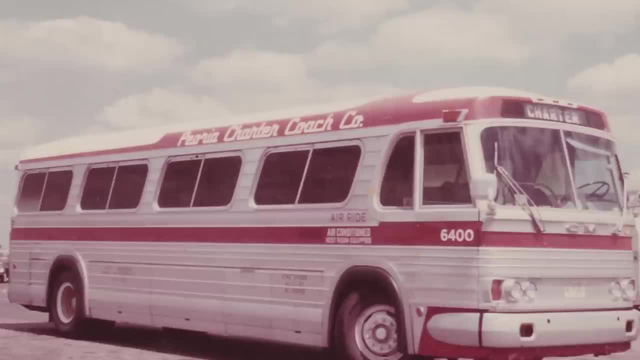 to ask him the real reason, And Roger replied that his father, Walter Winkler, the founder of Peoria Charter, made the change because the four-digit fleet numbers that denoted the year of when the vehicle was made were causing problems, because at some point his 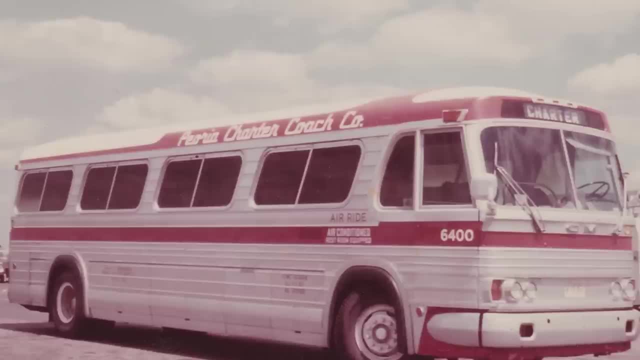 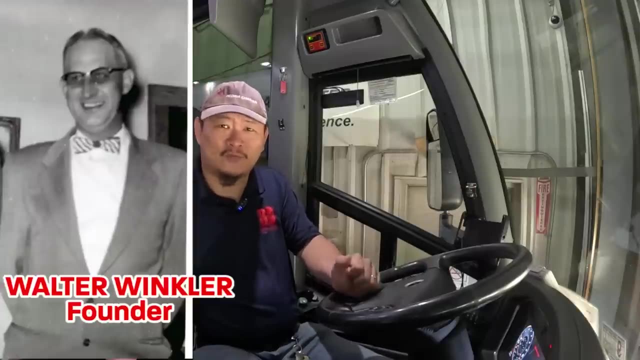 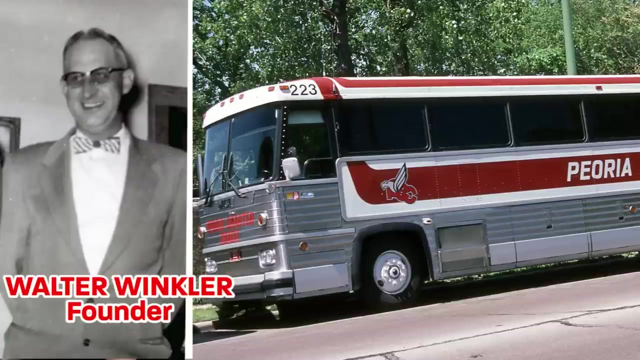 clients and passengers figured it out and started complaining when they realized they were on an older bus. Lesson learned right there. Well, Roger said that his father, Walt Winkler, chose to start each bus with a number two. after that, Well, two just happened to be his favorite number. 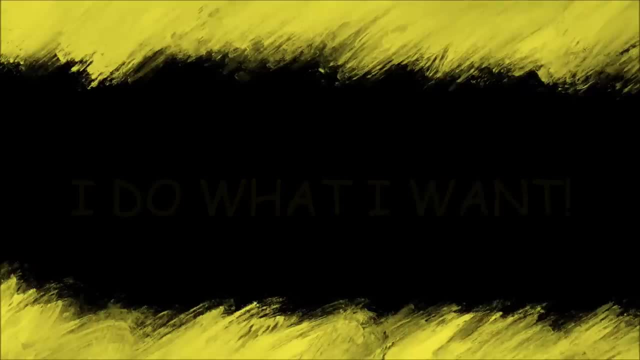 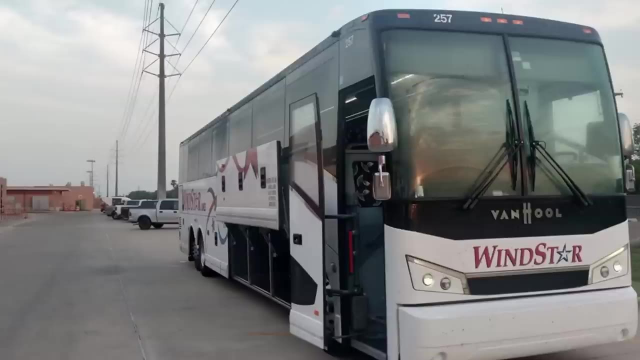 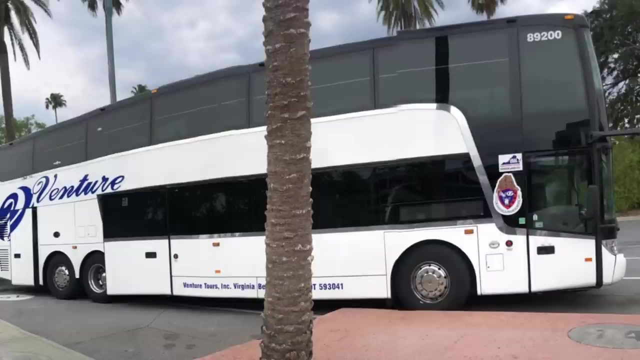 Now, when it comes to other privately owned motor coach companies, choosing their fleet numbers is completely up to them. Some buses are numbered by their owners based on the sequence of their purchase. Now I've actually seen some companies that number their buses based on the size of the. 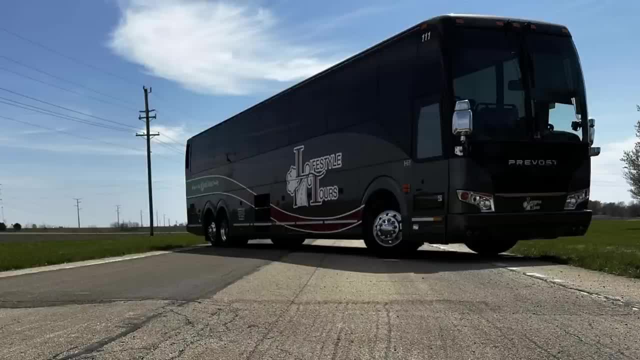 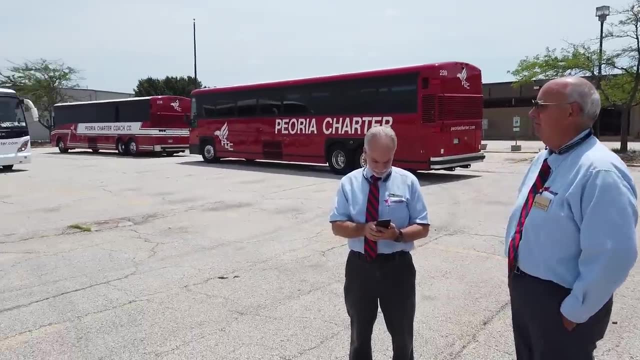 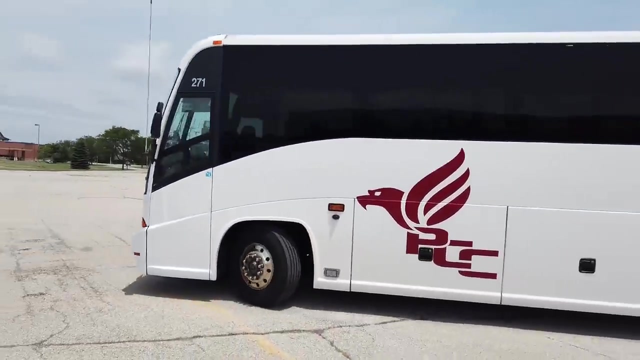 vehicle, with the number four denoting that they are 40 to 45 feet long, and their smaller vehicles. So starting with the number one. Now, despite whatever number a bus is assigned by the owners or the company, some buses are given unofficial names by the drivers that drive them or the company employees that interact. 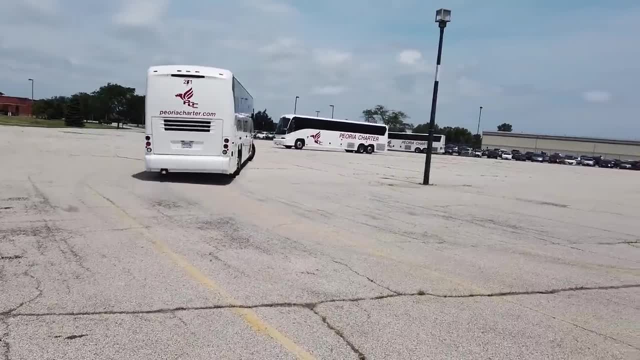 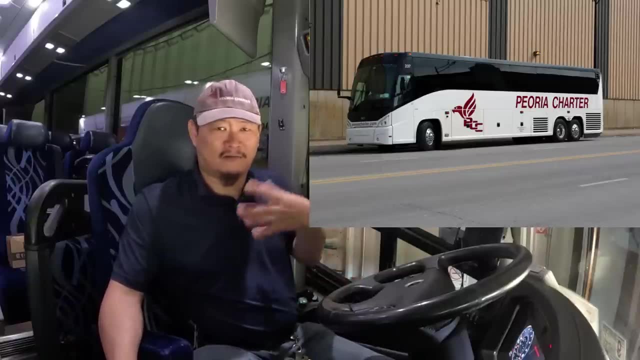 or work on them, sometimes due to their quirks or characteristics. Now you may ask: instead of giving them fleet numbers, why not just use their original VIN numbers? I mean, they're already unique and they're already there. And I will say: there are times when I'm selling one of our buses or dealing with banks and 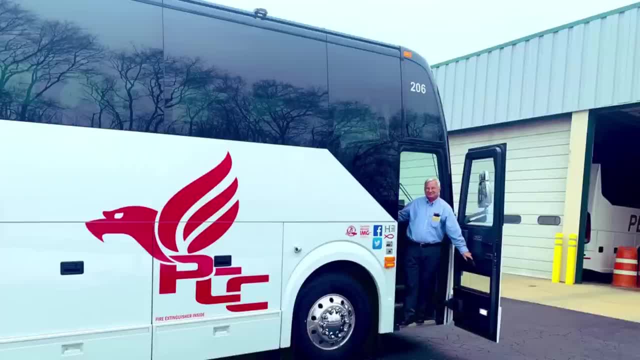 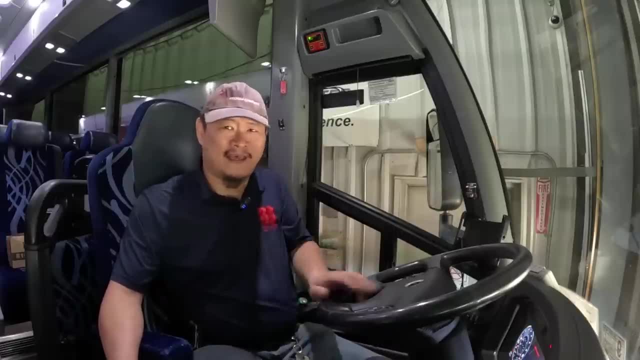 appraisers. the fleet numbers that we assign to our buses mean absolutely nothing to them. All they want are the actual VIN numbers. But I got to say that would be absolute hell on drivers, dispatchers and technicians if all we used were the VIN numbers. 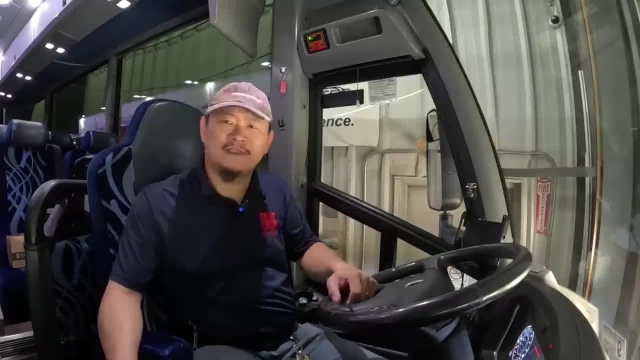 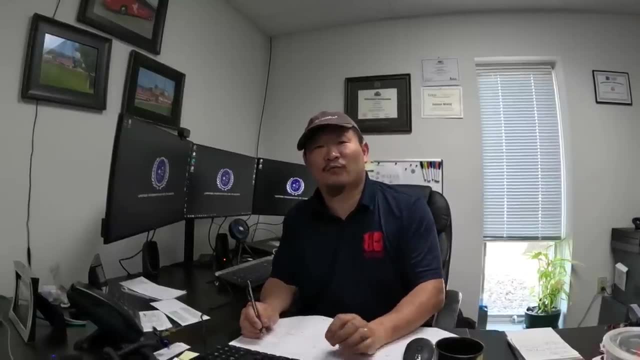 It's so much easier to say: hey, Bob, you're driving 203 today, 270 has to go in the shop. Can you imagine using a VIN number in this situation? Hey Leon, I'm putting you an E2XC81B6K3081419 today. 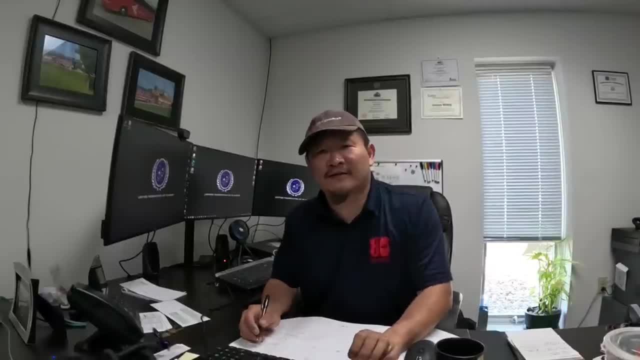 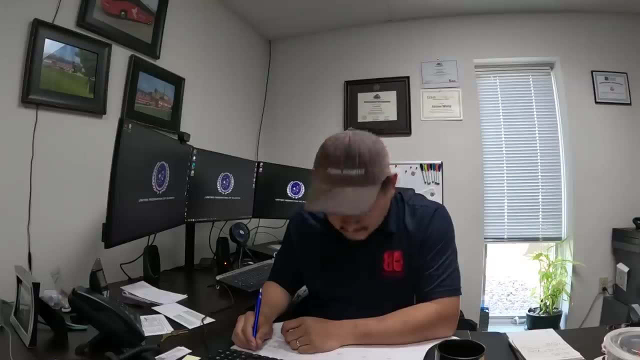 I'm going to give you a VIN number. I'm going to give you a VIN number. Your other bus, 2PCH33490PC721362, is in the shop. Which bus? Yeah, that's going to cause some delays. 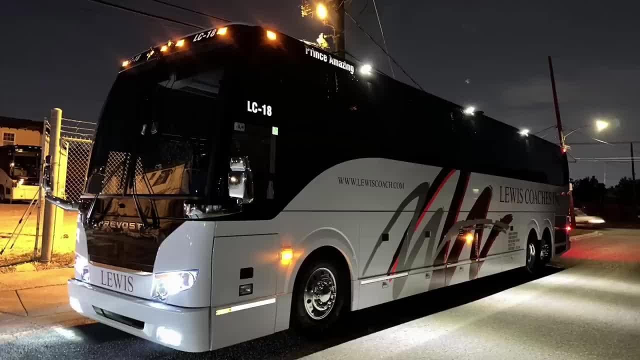 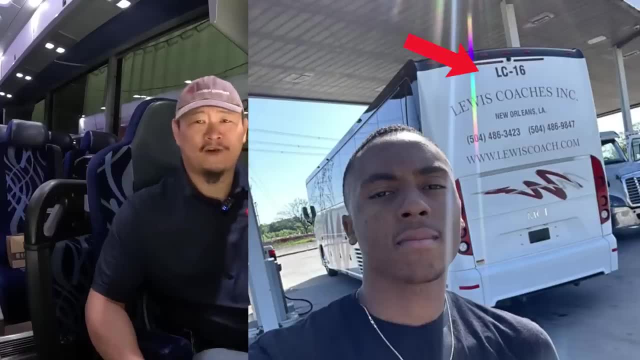 Now, one of my favorite examples is Lewis Coaches, Incorporated out of New Orleans. They identify their coaches with the two letters LC- which I'm assuming stands for Lewis Coach- followed by a dash and then a two digit number. On top of that, they also seem to give each of their coaches a number. 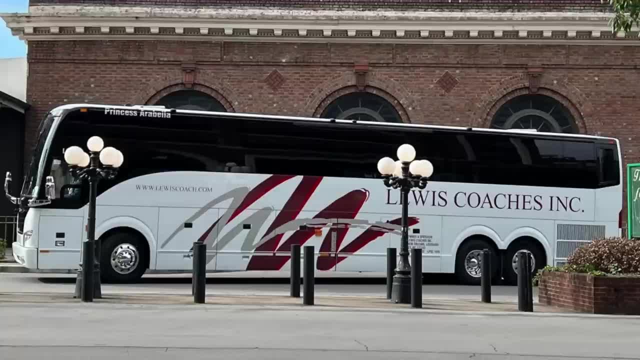 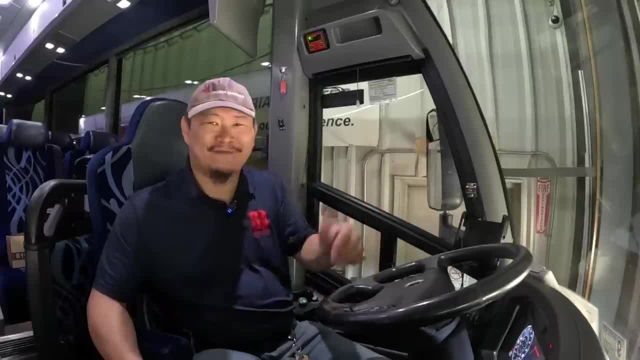 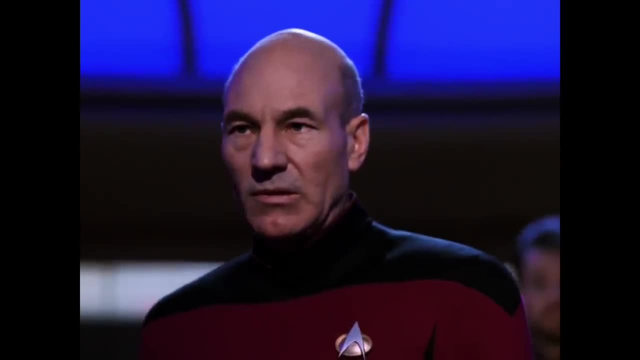 That's a name as well, like this one LC17,, which apparently is also known as Princess Arabella. Now, I don't know about you, but I think that's really cool that they actually give their coach buses names. Let's make sure history never forgets the name Enterprise. 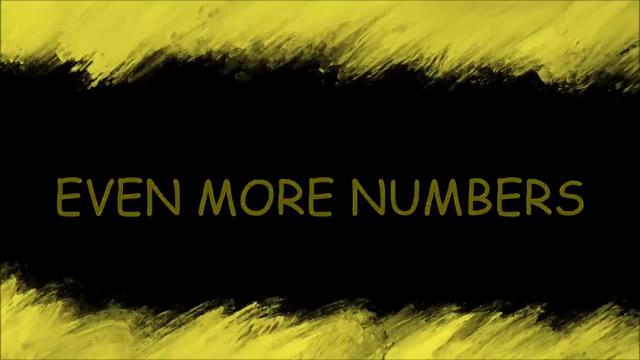 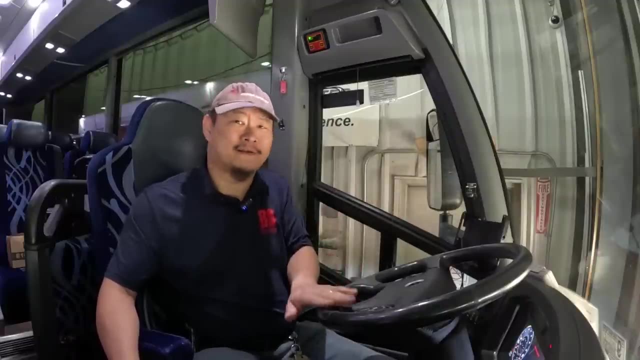 OK, if that wasn't enough numbers on a bus, well, there are situations where there could be even more. I mean, some of these buses, Some of these buses have more numbers than a Hong Kong phone book. What the hell you say? 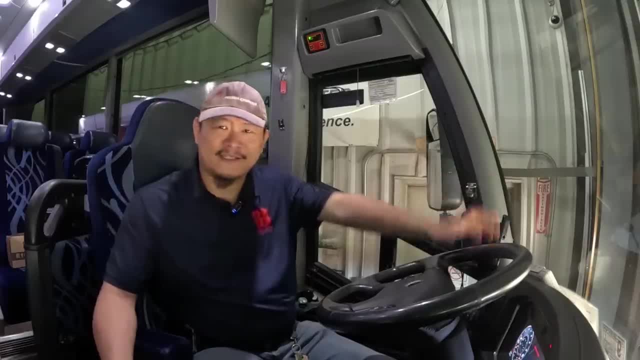 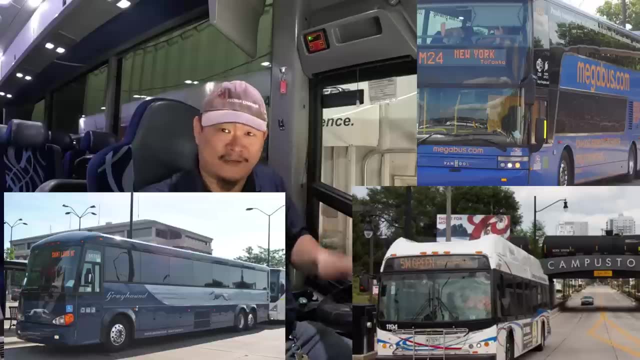 You know, I'm not sure why I used Hong Kong for that example. Population density maybe. Well, anyway, when it comes to motor coaches that operate line runs like Greyhound and Megabus or even city transit buses, there are even more numbers that they have to worry. 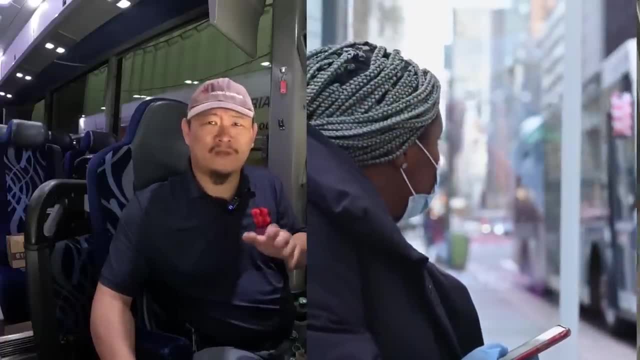 about. Well, if you're a passenger waiting for your bus to arrive, you probably won't even notice or care about any of the numbers or identifiers that I've mentioned so far in this video. The numbers and identifiers that the passengers are using are the same numbers that the bus. 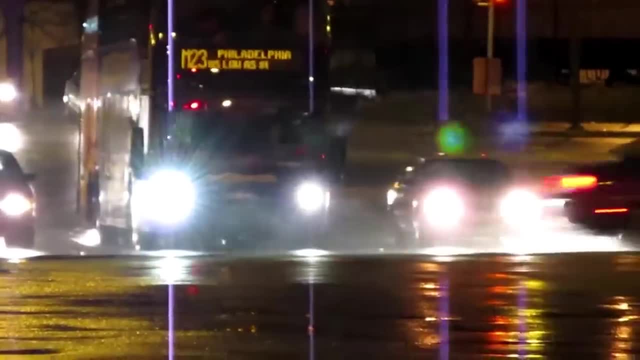 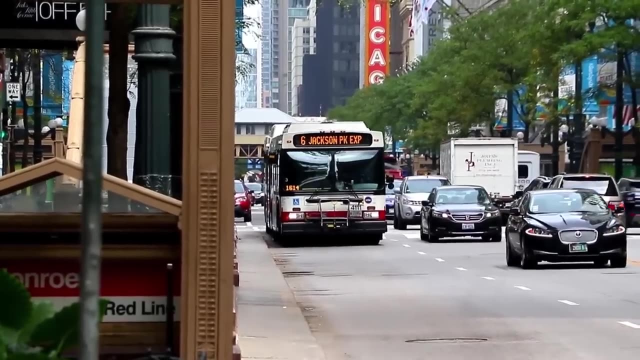 is using. The ones that the passengers are really focused on will be the destination marquees. They're usually illuminated and have a route number or name that define the route that this bus travels on. In Urbana, Illinois, the town that I live in, the local city transit agency known as 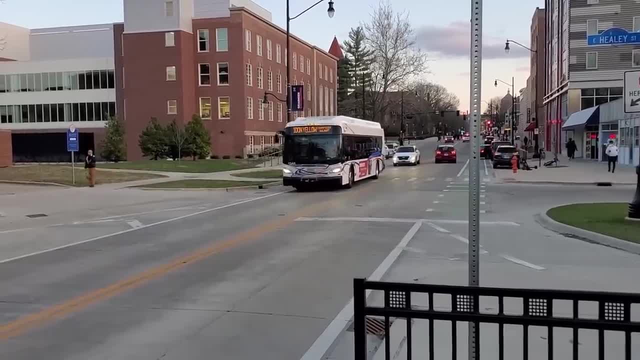 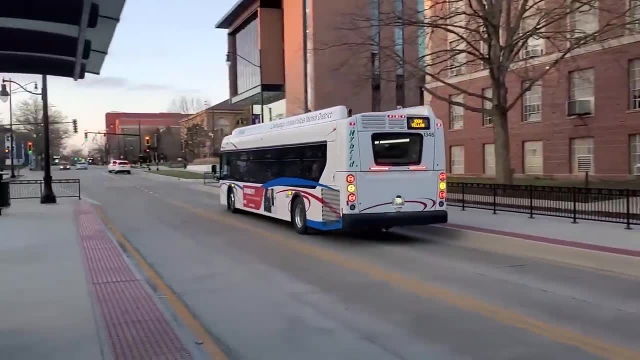 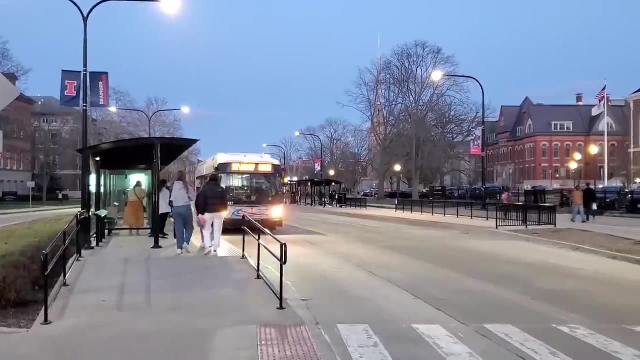 MTD uses names of colors that show what route the bus is operating. And, speaking of MTD, their buses actually use a four digit identifier for their fleet number And the first two numbers of that four digit number. actually, I wonder if they ever get any complaints from bus riders. that's figured out their numbering. 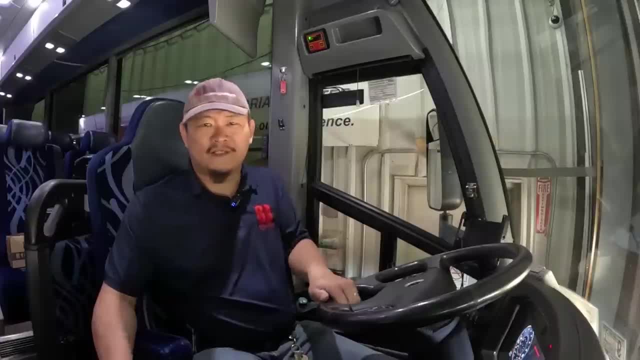 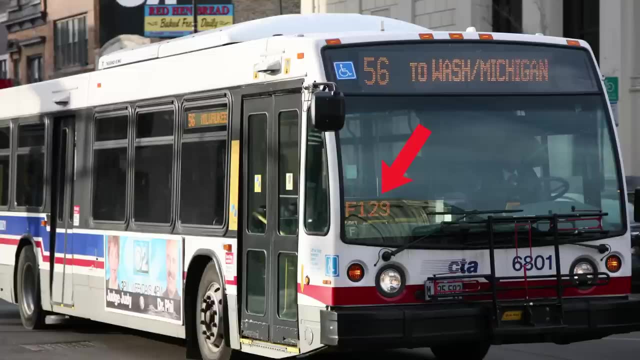 system and realized that their bus was kind of an old one. Some city transit buses have an additional illuminated sign on the bottom of the passenger side windshield, like the CTA buses in Chicago. Now, someone once told me that this was the run number, or some of them show the bus drivers. 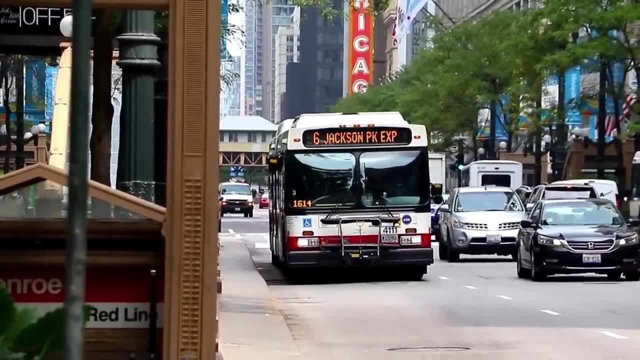 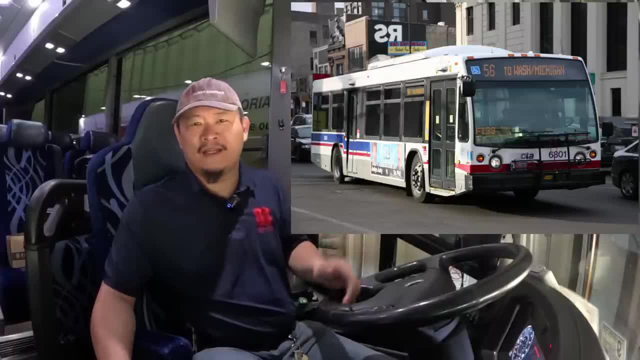 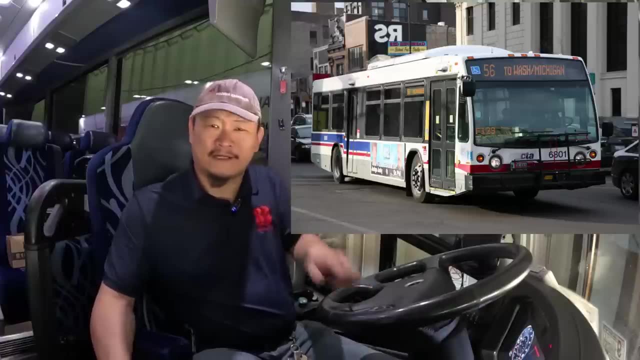 operator number on this little sign, So I guess bus drivers get their own unique numbers too. I don't know, But honestly I looked all over the place on the internet and I couldn't find any info on what that little display actually indicates, and it might be different between different. 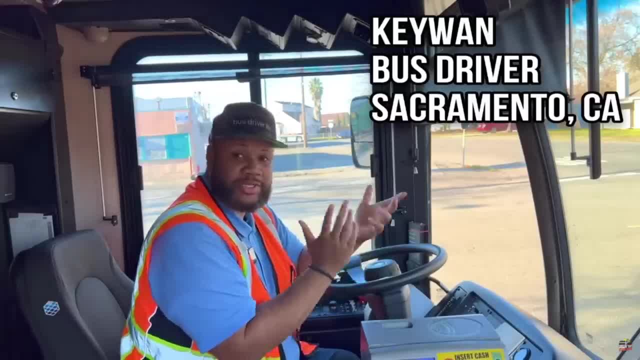 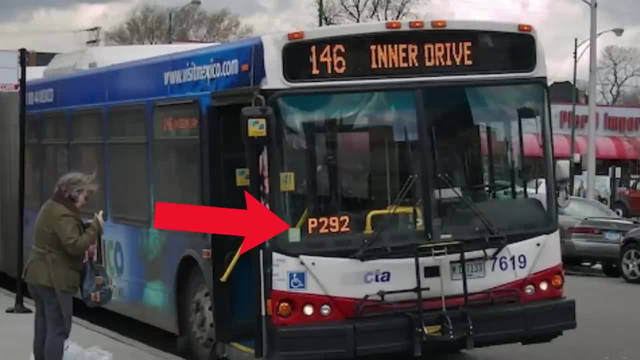 municipal transit agencies. Now, if any of you city bus operators or aficionados that are watching, could let me know what that sign actually displays down in the comments below, I would be most grateful. And finally, when it comes to school buses, most of them that I've ever ridden on as a 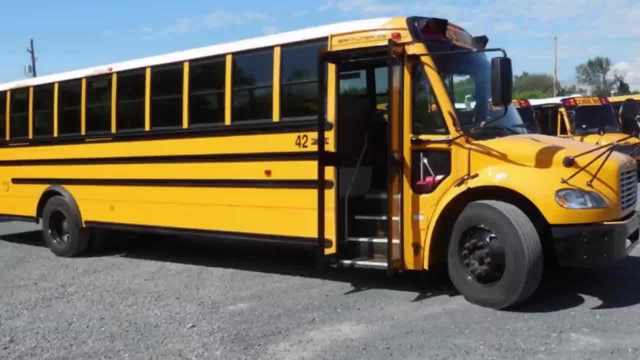 kid, as well as seen operating Have a simple two digit number on the side, and that number functions as the fleet number as well as the route number for all the kids that are boarding the bus. In larger cities, I've seen school buses with three or four digit numbers, as well as some